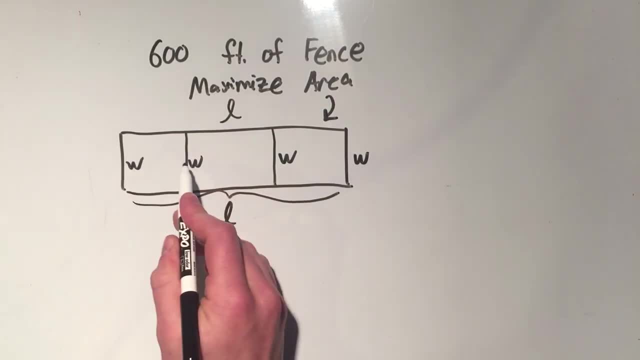 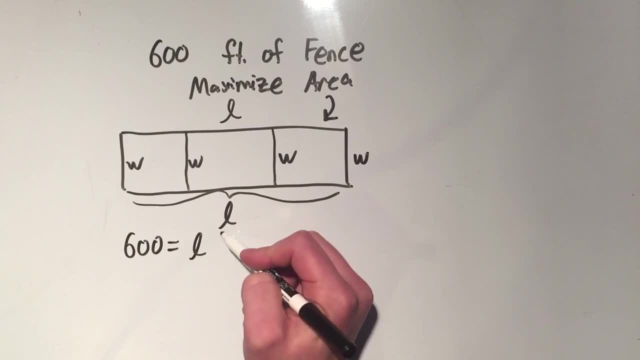 So I have 600 equals this L plus this L plus the first W plus the second W plus the third and the fourth, Or, if you like, L plus L is two L W four times is two L, And I might as well divide both sides by two, just to make it a little bit cleaner. 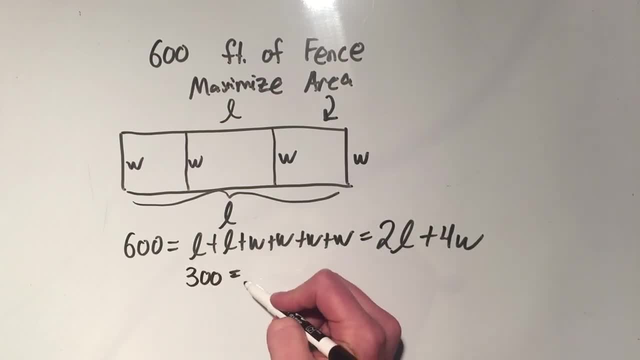 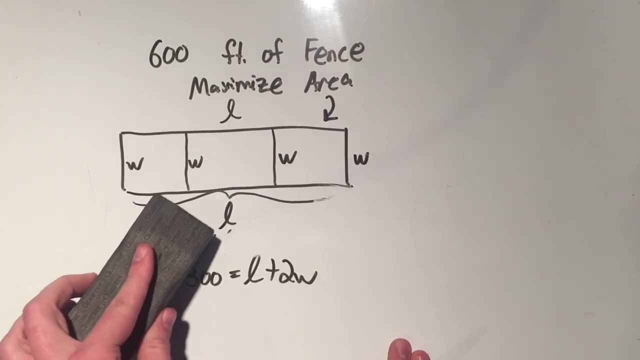 600 divided by two is 300.. Two L divided by two is L. Four L or four W divided by two is two W. Okay, So I have a nice neat little equation that describes my constraint. Your constraint is the number that you're given. So I only have 600 feet of fence. 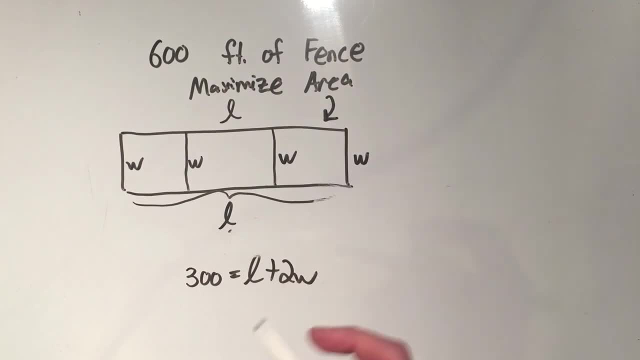 I'm constrained. I can't go out buy more fence. That's all I've got to work with. Maybe he's not a wealthy farmer, I don't know. I want to maximize the area. What's the area of this pen? 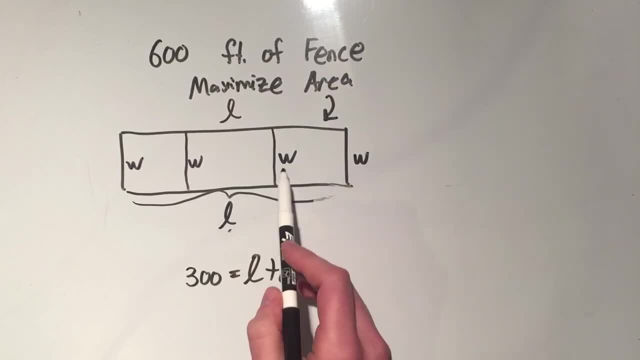 Well, as you know, the area of a rectangle is length times width. It doesn't matter that I've got these extra fences in there, Let's just assume that they don't really take away from the area. So the area, as we all know, I'm going to write up here. 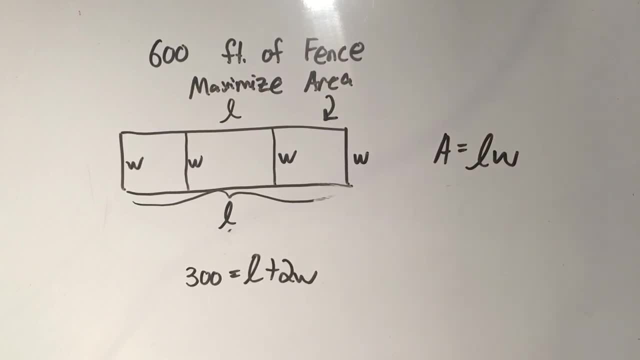 A for area is length times width. Now, this is the thing I want to take the derivative of, because it's what I want to maximize. This is the thing I want to take, I'm sorry, This is the thing I want to maximize. 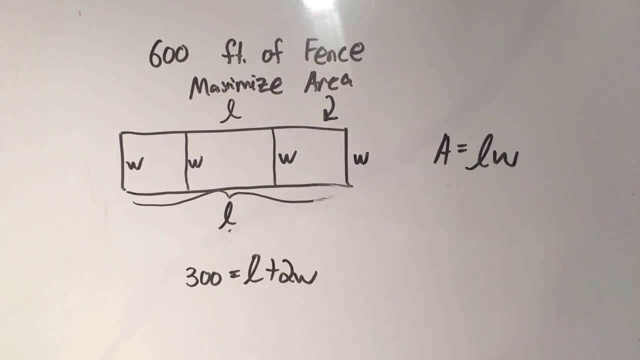 This is the thing I want to take the derivative of, But it's in terms of two variables. I don't feel like doing a product rule, I don't feel like doing an implicit differentiation kind of deal. So let's use what we already know about L and W and we're going to make a substitution. 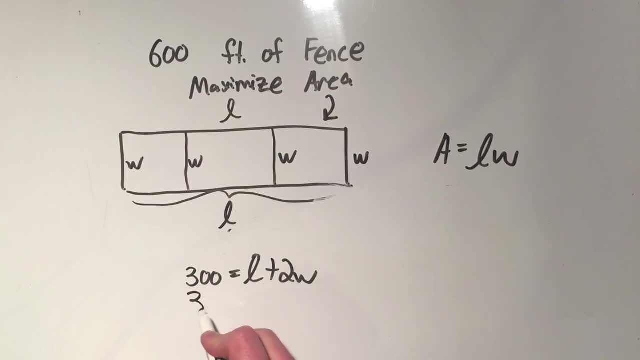 You'll see That if I subtract two W from both sides of this equation, I'll have 300 minus two W equals L, And now I have an expression in terms of an expression of L, in terms of just W, And now I'm going to substitute that in for this L in my area equation. 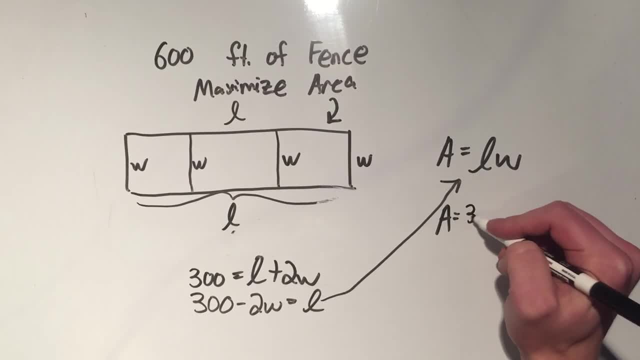 So I have area equals length times width. But now that we know, L is 300 minus two W times W, And if I distribute that I'll have 300 W minus two W squared. Now my area is in terms of just W, which means I can take the derivative of both sides. 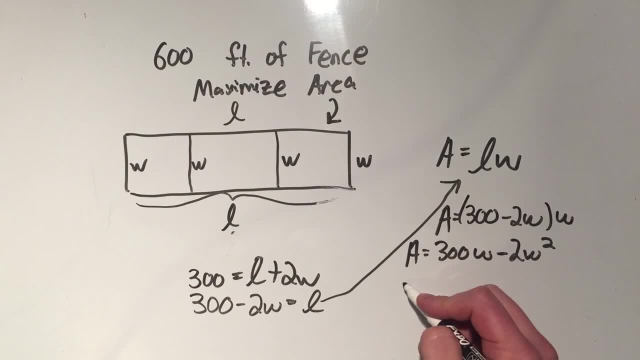 Well, area, the area of this thing is just a constant right. The derivative of a constant is zero. The derivative of 300 W is 300.. The derivative of minus two W is zero And the derivative of minus two W squared is minus four W. 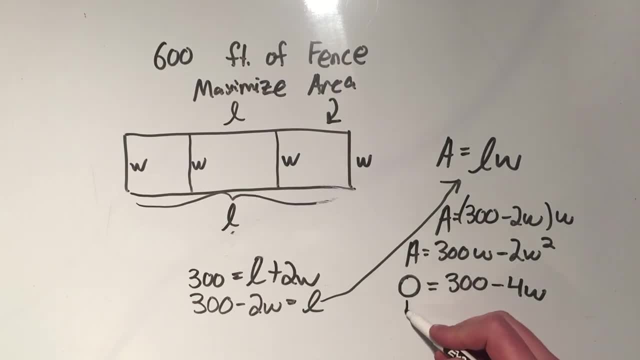 And hey, look at this. I have a really simple equation to solve. If I just add four W to both sides, four W equals 300.. Divide both sides by four, I'm getting W equals 300 over four. I think it's going to be 150 over two is going to be 75.. 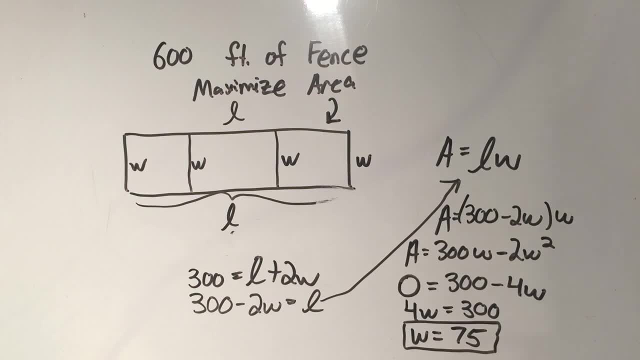 I have that W equals 75. Now that I know what W is, I can take that value and substitute it in for L. And if I substitute it in for my W in my L equation I'll have 300 minus two W. 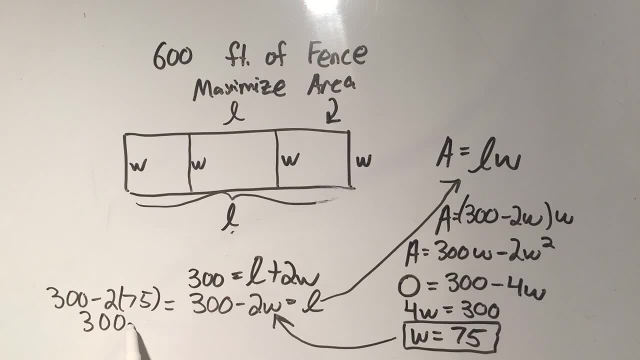 W is 75.. Two times 75 is 150.. 300 minus 150 is 150.. So that means my pen, to have maximum area, has to have a length of 150 and a width of 75. And if I actually want the area, 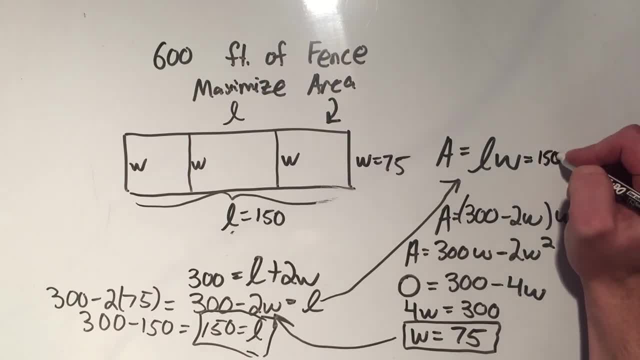 the area that is maximized. I'll multiply those two things together. I'll do length times width, And this is the point where I am thoroughly unprepared because I did not calculate this value. So whatever 100 times 75 is will be the maximum area. 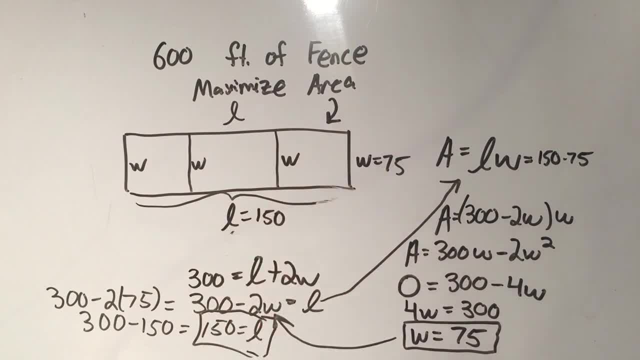 So the whole name of the game here is: I like to draw a picture and label it. You use your constraint to set up an equation And then the other equation is whatever you want to maximize or minimize. You solve for one of the variables in the constraint equation.